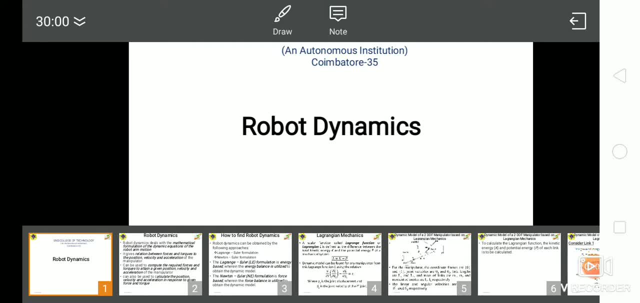 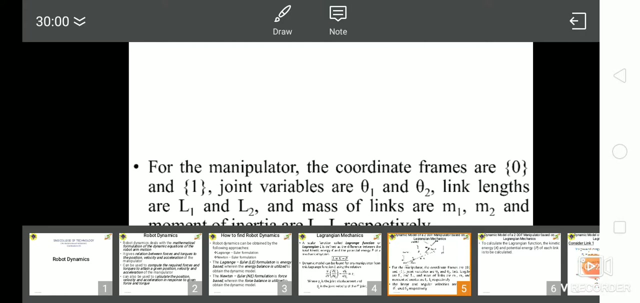 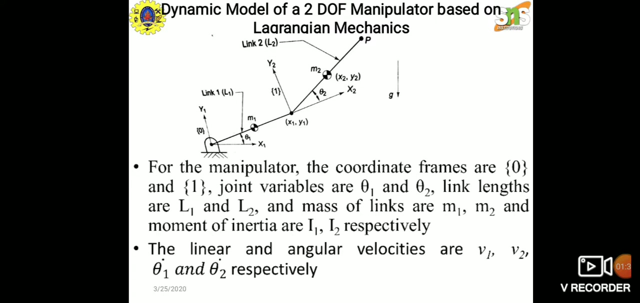 The Lagrange-Euler formulation. LE is energy based, wherein the energy balance is utilized to obtain the dynamic model. Next one is Newton-Euler energy formulation. It is a force to obtain the dynamic model, Lagrange mechanics. we call it as Lagrange function or Lagrange. 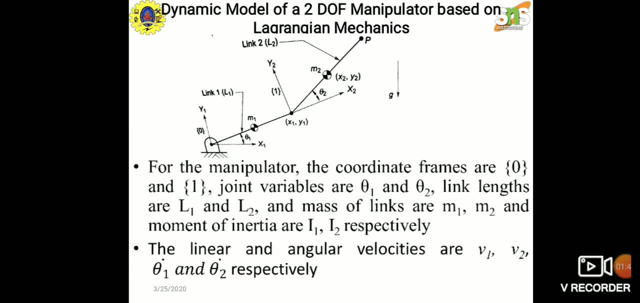 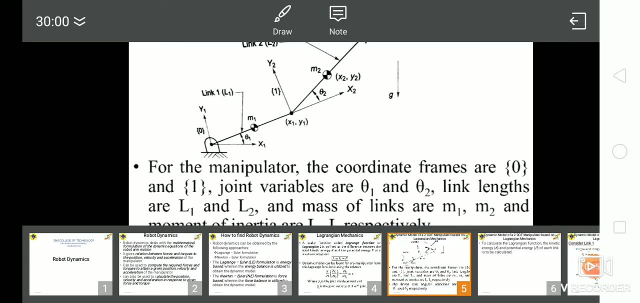 L. Here the L is defined as the difference between the total kinetic energy K and the potential energy P of a mechanical system, L equal to K minus P. The dynamic model can be found for any manipulator from this Lagrange-Euler function L using the: 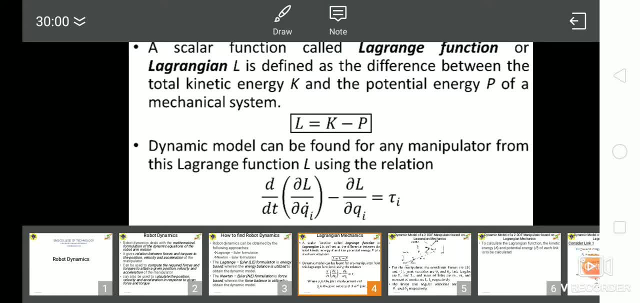 equation D by DT multiplied with dou L by dou Qi dot, minus dou L by dou Qi, equal to tau I, where Q is the joint displacement and Qi dot is the joint velocity of the I-th joint. OK, We are going to discuss about dynamic model of a 2D wave manipulator based on Lagrange. 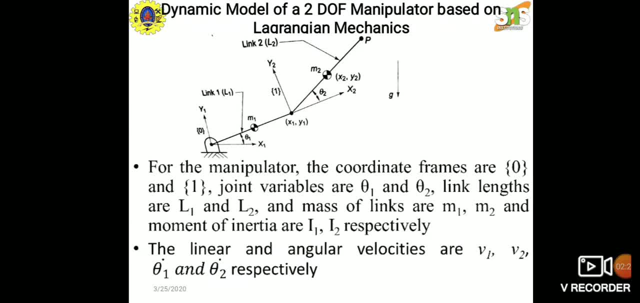 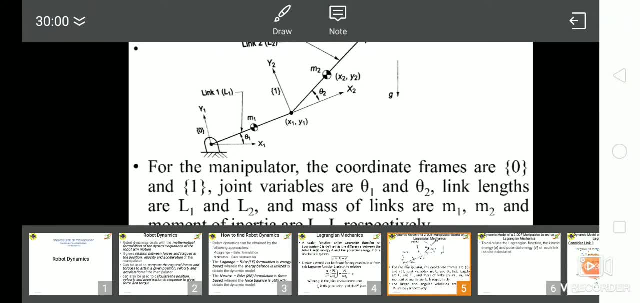 mechanics: 4., 1., 2., 5.. For the manipulator, the coordinate frames are 0 and 1 and the joint variables are theta 1 and theta 2.. The link lengths are L1 and L2 and most of the links are M1, M2 and moment of inertia are I1, I2 respectively. 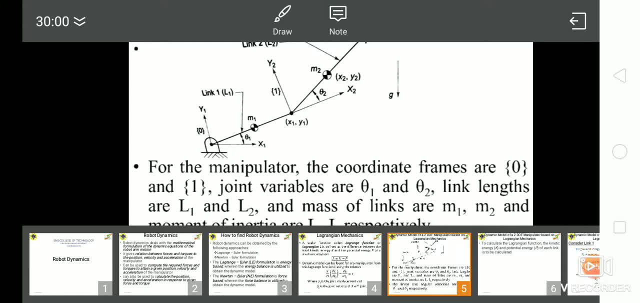 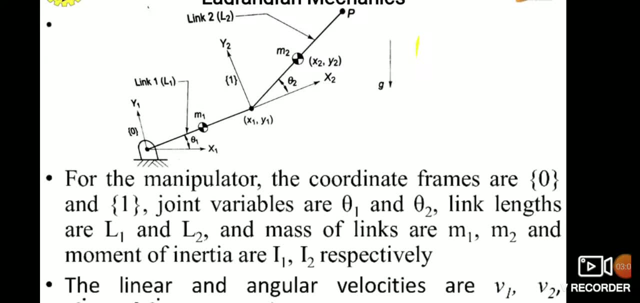 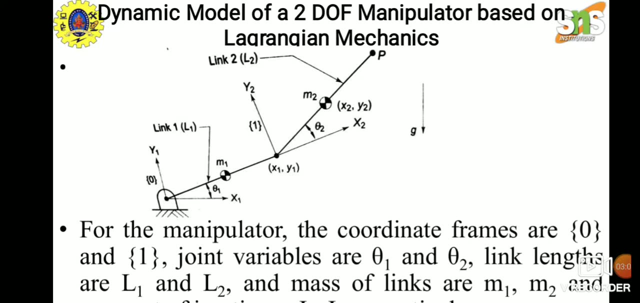 Here the linear velocities are V1, V2 and angular velocities are theta 1 dot and theta 2 dot. Here we have two links: L1 and L2.. The coordinate frames are already. we have seen the 0 and 1.. Here the joint variables are theta 1 and theta 2.. 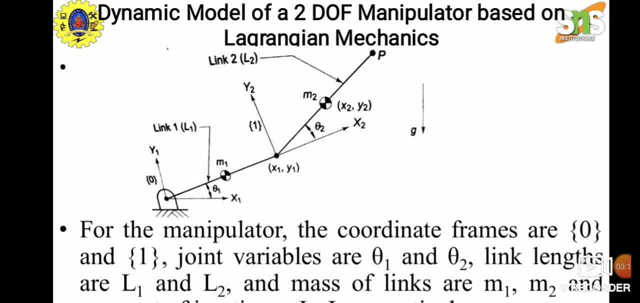 For link 1, it is theta 1, for link 2 it is theta 2.. Most of the links for link 1 is M1, for link 2, M2.. Why do we use X and Y here? Because we use Cartesian coordinate systems. 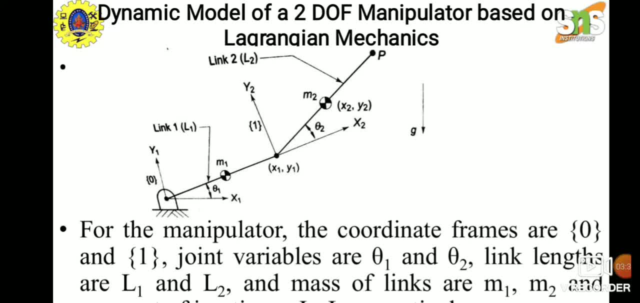 So it is X1, Y1 for link 1, X2, Y2 for link 2.. And also we have two velocities: linear and angular velocities. Linear velocity for link 1 is V1, for link 2 it is V2.. 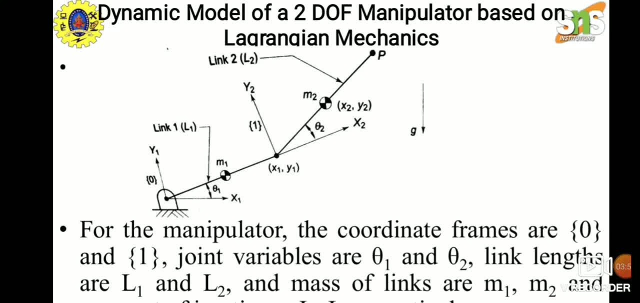 Angular velocity for link 1 is theta 1 dot and for link 2 it is theta 2.. To calculate the Lagrangian function, the kinetic energy K and the potential energy P of each link is to be calculated Because L equal to K minus P in Lagrangian Euler formulation. 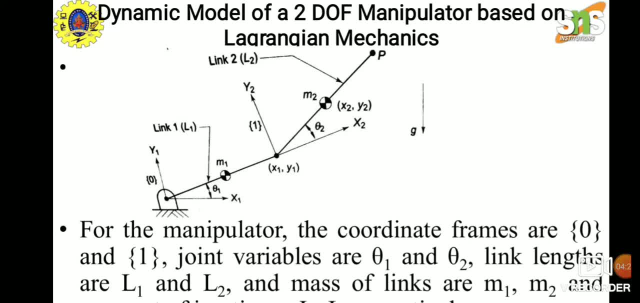 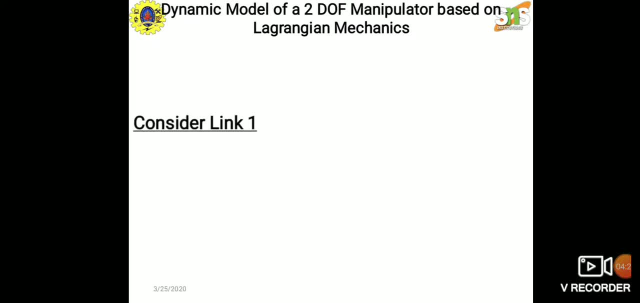 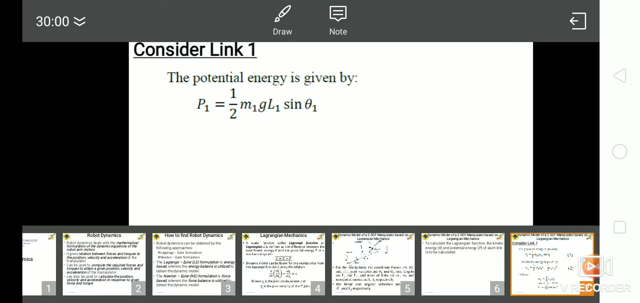 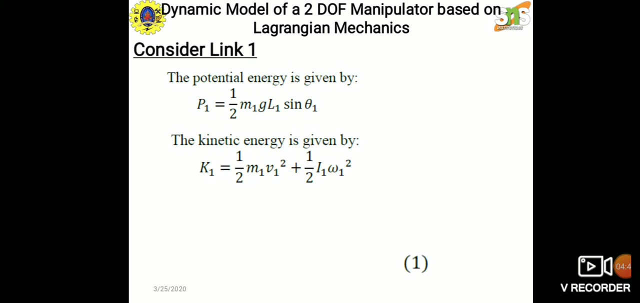 For in this we have two links. First, consider link 1.. consider link one. here the potential energy is given by p1, equal to 1 by 2 m1 g l1 sine theta 1. the kinetic energy is given by k1: 1 by 2 m1 v1 square plus 1 by 2 i1 omega 1 square. 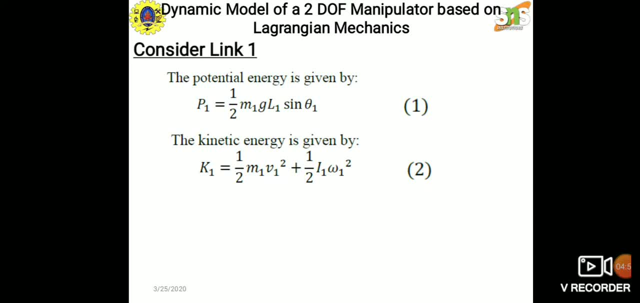 let us consider as equation 1 and equation 2, where v1 equal to 1 by 2 l1 theta 1 dot, omega 1 equal to theta 1 dot and i1 equal to 1 by 12 m1 l1 square. here p represents potential energy. 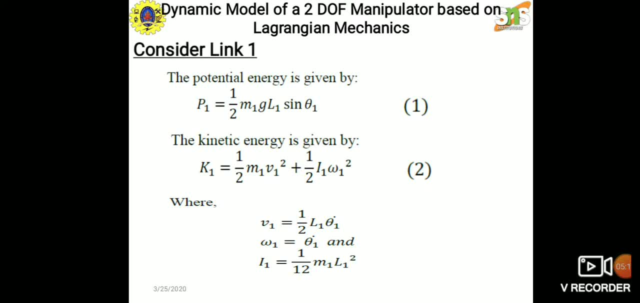 k is kinetic energy, p1 is potential energy for link one, k1 is kinetic energy for link one. so ms represents mass. next g is gravity: l1 for link one. length of link one. sine theta 1 for link one. linear angular velocity of link one. here the linear velocity is b1 and b2. 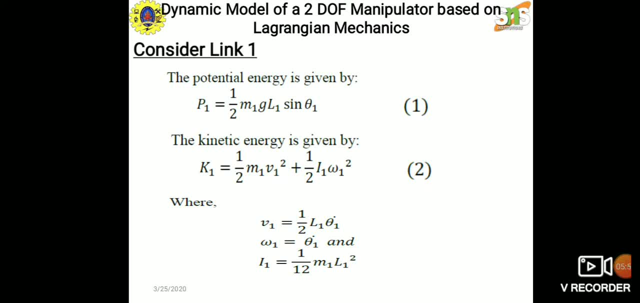 substituting the values of ms represents mass. next, g is gravity. l1 for link one. length of link one sine. theta 1 for link one. linear angular velocity of link one: here the linear velocity is b1 and b2, V1,, omega 1 and I1, we can get k1 equal to 1 by 6 m1 l1 square. theta 1: dot whole square. 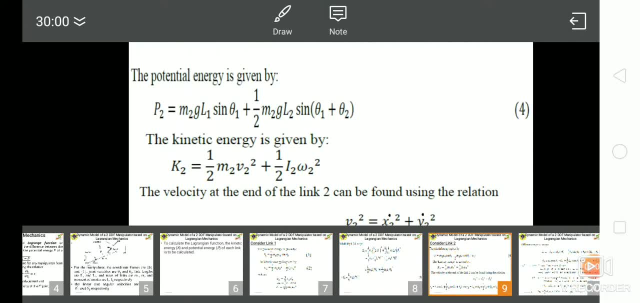 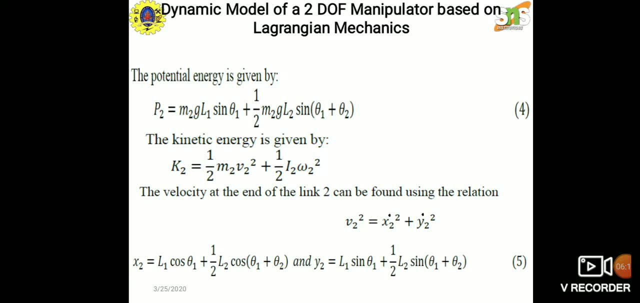 Next for considering link 2, we can get p2 equal to m2 g l1 sine theta 1 plus 1 by 2 m2 g l2 sine theta 1 plus theta 2.. Here the kinetic energy is k2 equal to 1 by 2 m2 v2. 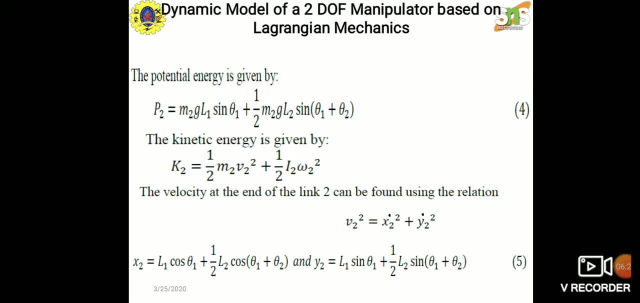 square plus 1 by 2, I2, omega 2, the whole square. Here the velocity at the end of the link 2 can be found using the relation: v2 square equal to x2 dot square plus y2 dot, the whole square. We know that x2 equal to l1 cos theta 1 plus 1 by 2, l2 cos theta 1 plus theta 2. 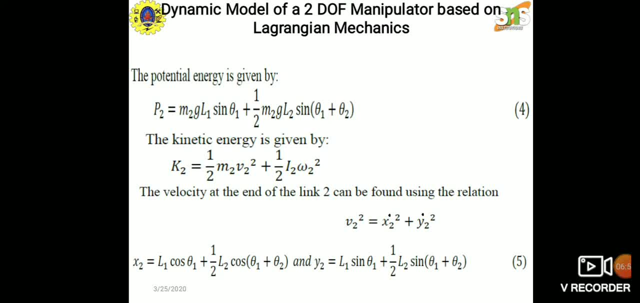 and y2 equal to m2 g l2 sine theta 1 plus theta 2.. Here the kinetic energy is k2 equal to l1 sine theta 1 plus 1, by 2 l2 sine theta 1 plus theta 2.. Differentiating x2 and y2, we get minus l1 sine theta 1 multiplied with theta. 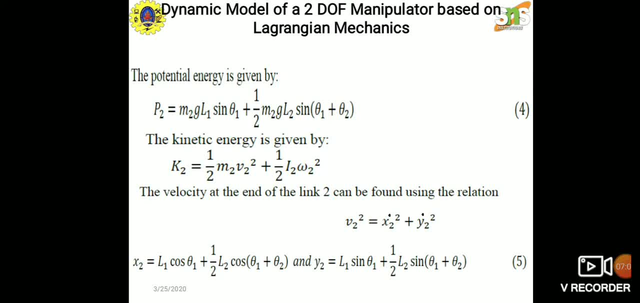 1 dot minus 1 by 2 l2 sine theta 1 plus theta 2, multiplied with theta 1 dot plus theta 2 dot, Here y2 dot equal to l1 cos theta 1 multiplied with theta 1 dot plus 1 by 2 l2 cos theta. 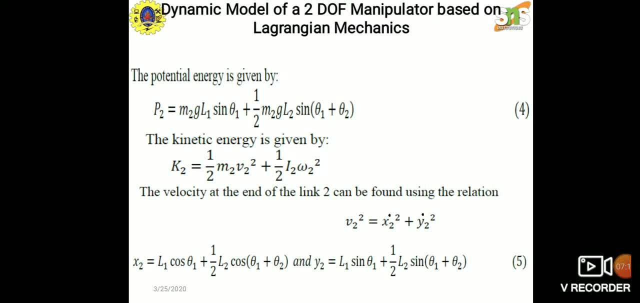 1 plus theta 2 multiplied with theta 2 dot. Here y2 dot equal to l1 cos theta 1 multiplied theta 1 dot plus theta 2 dot. Here omega 2 equal to theta 1 dot plus theta 2 dot. and. 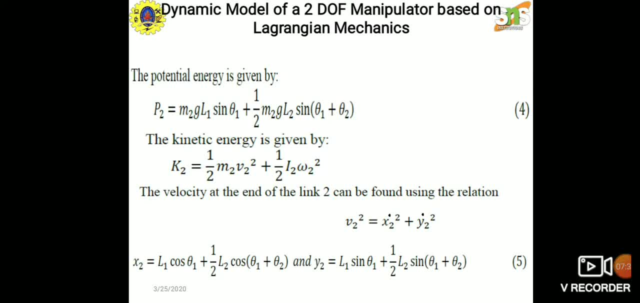 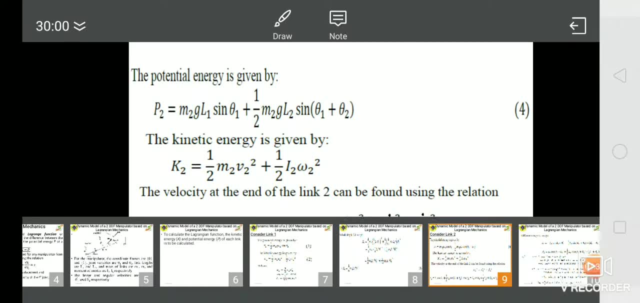 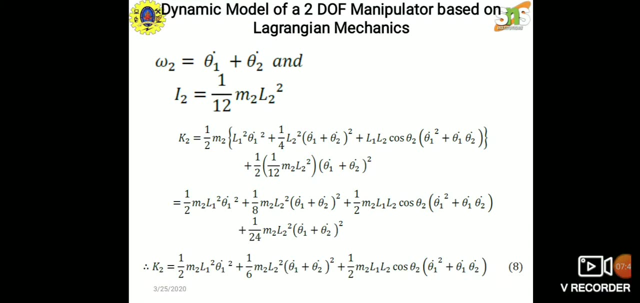 I2 equal to moment of inertia, 1 by 12 m2 l2 square for link 2.. So we calculate the kinetic energy for link 2 as 1 by 2 m2 l1 square- theta 1 dot square, plus 1 by 6 m2 l2 square- theta 1 dot. 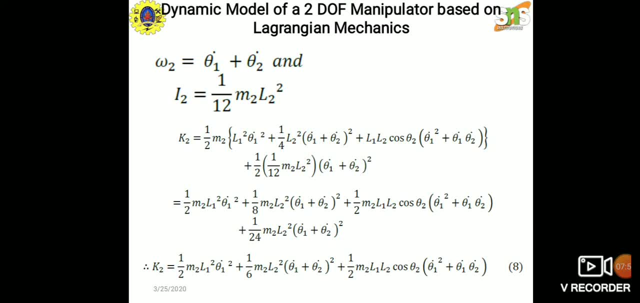 plus theta 2 dot, the whole square plus 1 by 2 m2 l1 l2 cos. theta 2 multiplied with theta 1 dot square plus theta 1 dot multiplied with theta 2 dot For link 1, we have k1 equal to 1 by 6. 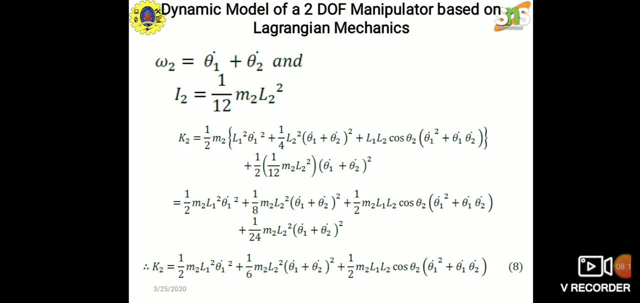 m1 l1 square. theta 1 dot square for link 2 k2 equal to 1 by 2 m2 l1 square. theta 1 dot square plus 1 by 6 m2 l2 square multiplied with theta 1 dot plus theta 2 dot plus 1 by 2 m2 l1 l2 cos. 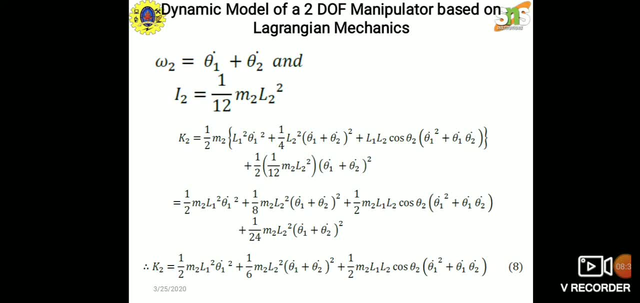 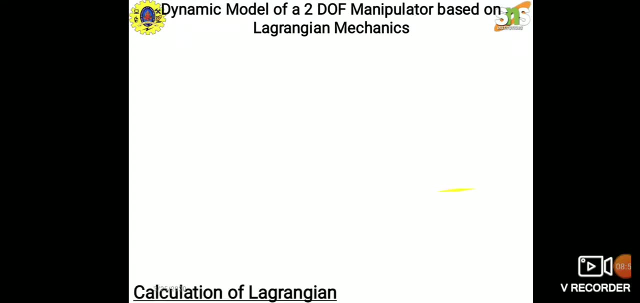 theta 2 multiplied with theta 1 dot. square plus theta 1 dot, theta 2 dot. So what's the time to calculate lagrangian? The lagrangian is given by l equal to k minus p. Here k equal to k1 plus k2 for link 1 and link 2.. p is p1 and p2, so k1 plus k2 minus p1 plus p2. 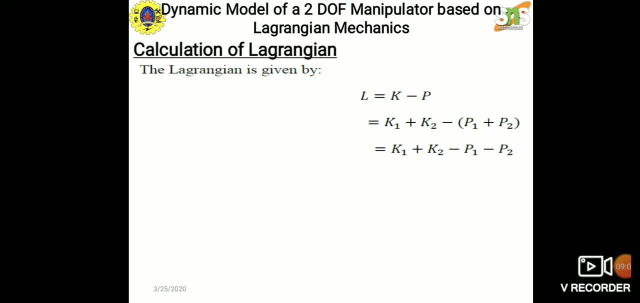 it is equal to k1 plus k2 minus p1 minus p2.. Substitute the lagrangian for k1 plus k2.. In the equations of k1, k2 and p1- p2, we can get l equal to 1 by 6 m1 l1 square. theta 1 dot square. 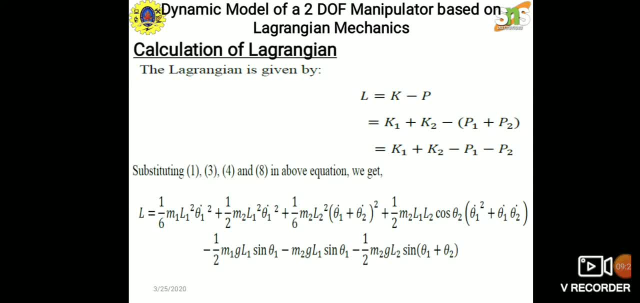 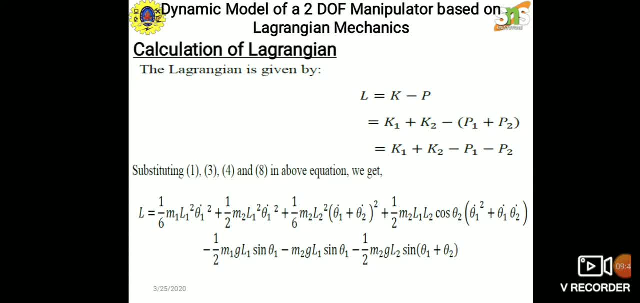 m2 l1 l2 cos theta 2 multiplied with theta 1 dot square plus theta 1 dot multiplied with theta 2 dot minus 1 by 2 m1 g l1 sin theta 1 minus m2 g l1 sin theta 1 minus 1 by 2 m2 g l2 sin theta 1. 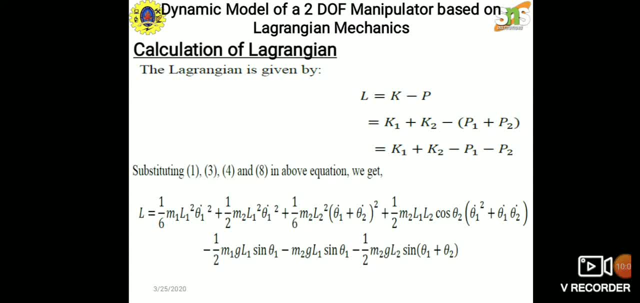 plus theta 2.. So from this we can extract the tau 1 equal to d by dt dou l by dou theta 1 dot minus dou l by dou theta 1.. Substituting the equations of l k1, k2, p1 k2 and p1 k2, we can get d by dt dou l by dou theta: 1 dot minus dou l by dou theta 1.. 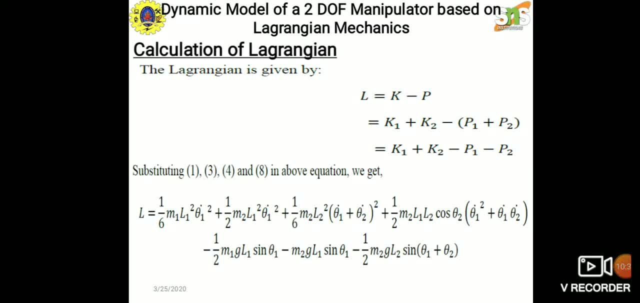 And p1 and p2, we can get the tax tau 1 and tau 2.. It represents the motion of 2d wave manipulator arm. It is also called as dynamic model of a 2d wave manipulator arm. It can be: 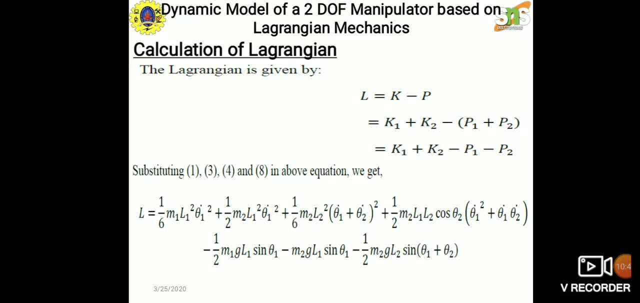 observed that this is technique is complex just for a simple 2d wave manipulator. Finding the dynamic model for higher d wave manipulator arm would be even more complex. Hence a generalist approach to this is not important. The device is only used for simple operations. Make sure that 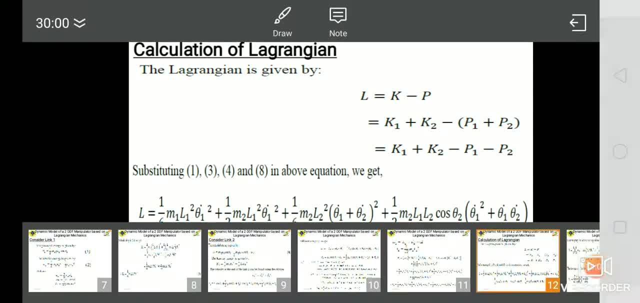 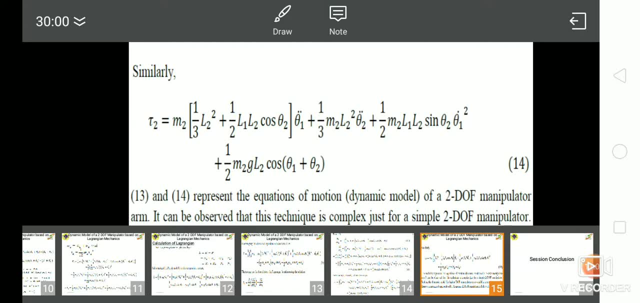 called Lagrange Euler formulation is followed. The Lagrange Euler formulation consists of eight steps. It is a systematic procedure for obtaining the dynamic model of an end-wave manipulator. This Lagrange Euler formulation establishes the relationship between joint positions, velocities, accelerations. 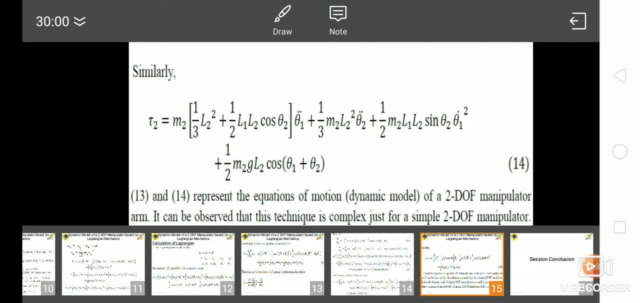 and the generalized tacks applied to the manipulator. The equations of the motion obtained are analytical and compact. Already we have seen the dynamic model of 2d wave manipulator as tau1 and tau2 in terms of L1, L2, K1, K2 and P1, P2.. 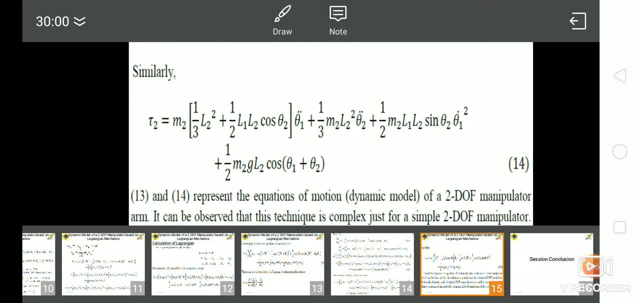 The matrix vector form of equations is appealing for calculations and control system design. The Lagrange Euler dynamic model algorithm consists of nine steps. Step 1 is assigning frames using Denavit-Hurtenberg notation. Step 2 is applying the link transformation matrix. Step 3 is considering a revolute or prismatic.